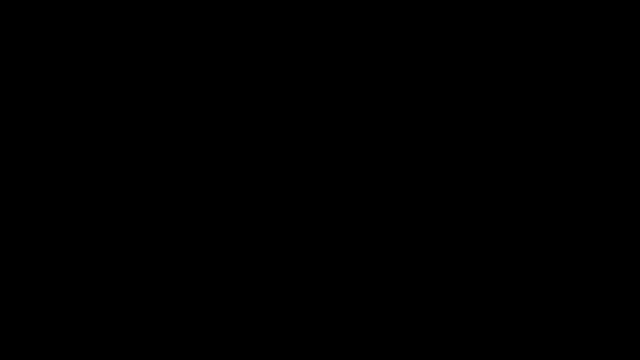 That is beautiful. One day I dream I can achieve that. Damn You know, that's not human Insanity. I don't even know what I just watched. I'm happy to see that in person. That is like: do you have a vision of what's coming? 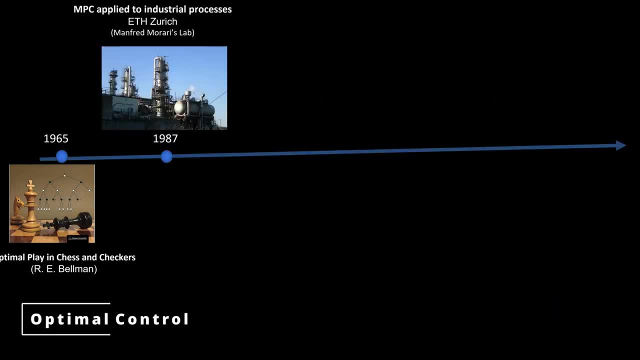 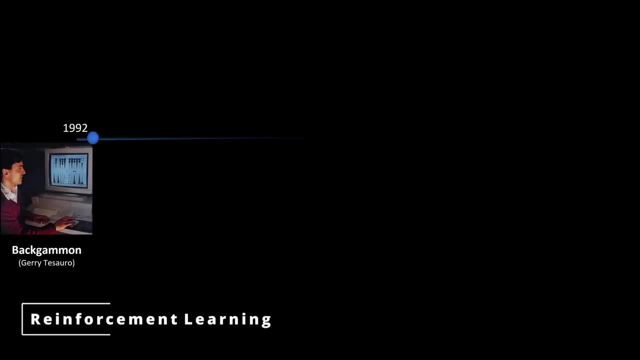 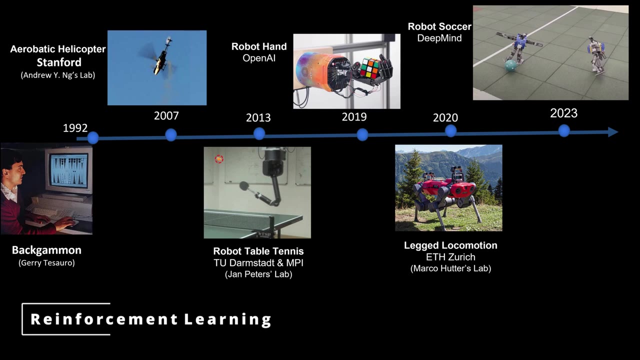 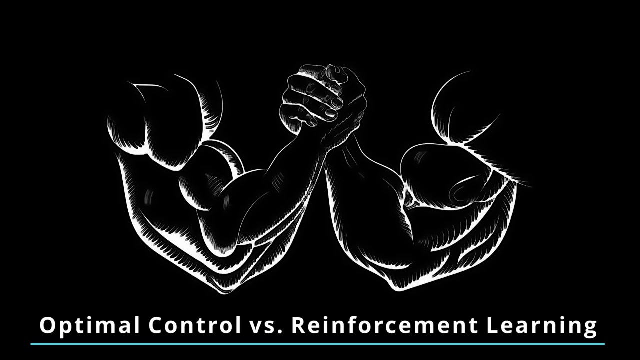 Optimal control has been successful in tackling control problems in fairly well-understood dynamical systems. Reinforcement learning has arisen as an attractive alternative to conventional controller design, achieving impressive performance in applications such as quadrupedal locomotion over challenging terrain. In this work, we study the fundamental factors that have led to the success of reinforcement learning. 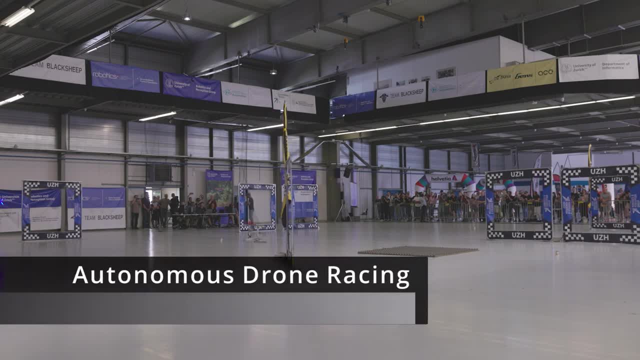 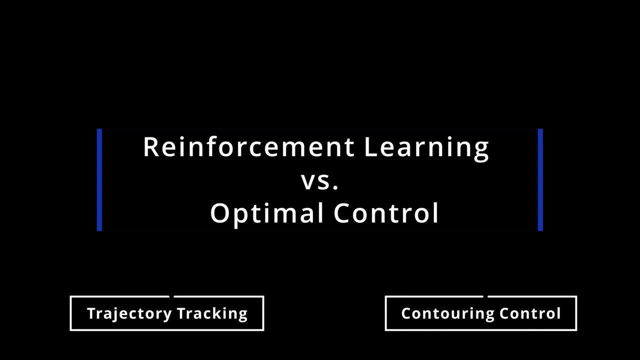 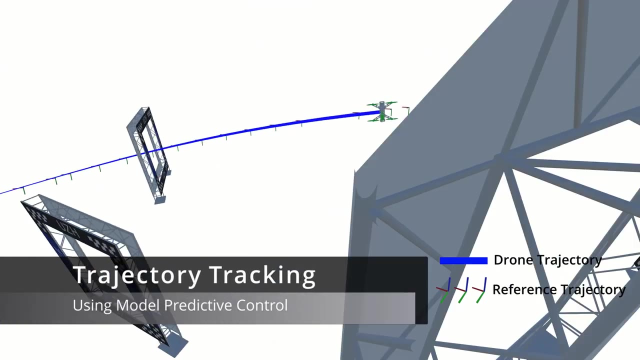 We focus on a challenging control problem: Autonomous drone racing. We compare the reinforcement learning policy against two state-of-the-art optimal control methods: trajectory tracking and contouring control. Trajectory tracking follows a pre-computed time-optimal trajectory using model predictive control. 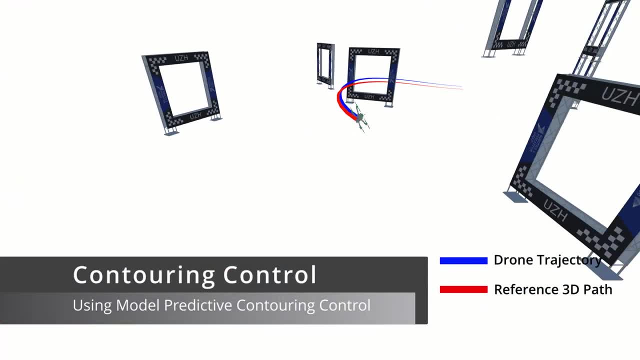 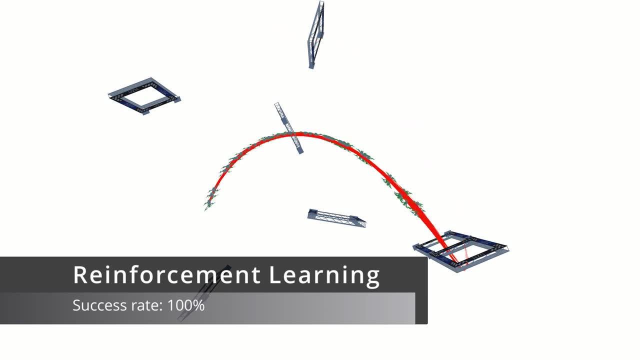 On the other hand, contouring control maximizes the progress along a reference path. In extensive experiments, the reinforcement learning policy significantly outperforms both optimal control methods, particularly when conditions at the test time are different from conditions during training. We now ask: what is responsible for the superior performance of reinforcement learning? 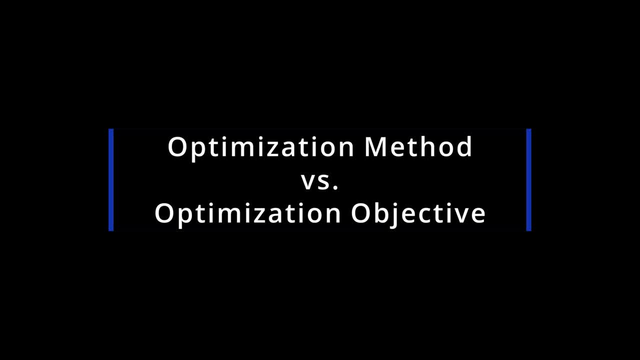 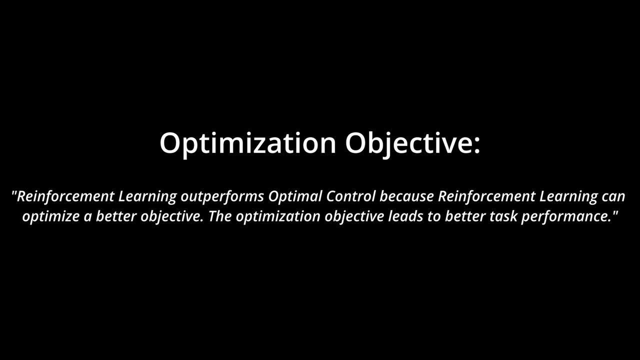 We study this question along two axes: the optimization method and the optimization objective. Our study indicates that reinforcement learning is necessary to achieve high performance. performance in training learning outperforms optimal control because reinforcement learning can optimize a better objective. The optimization objective leads to better 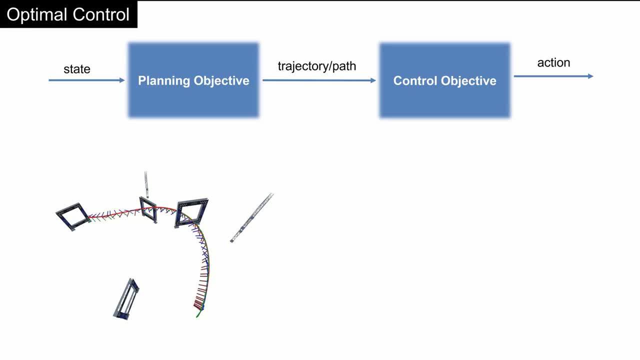 task performance. Optimal control imposes a decomposition of the problem into planning and control, with an explicit intermediate representation, such as a trajectory or a path that serves as an interface between the two layers. This decomposition limits the range of behaviors that can be expressed by the